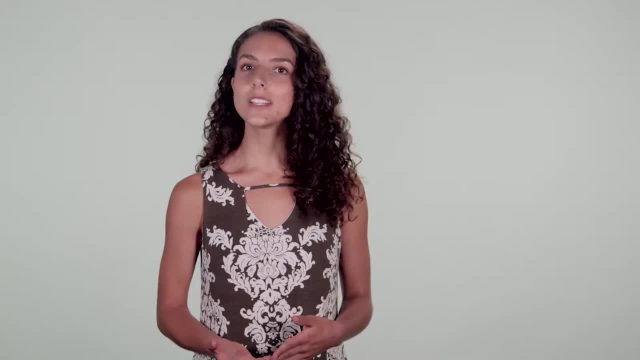 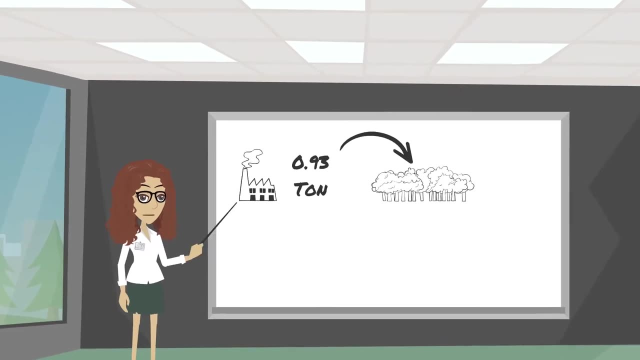 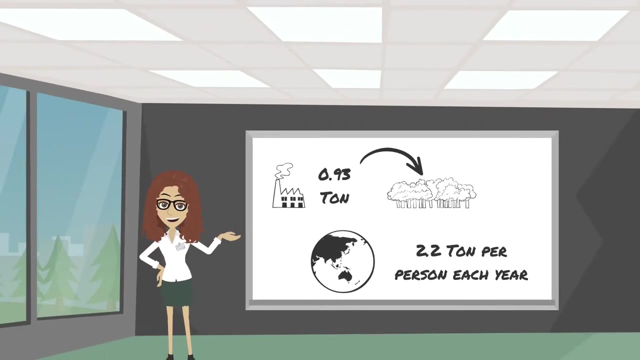 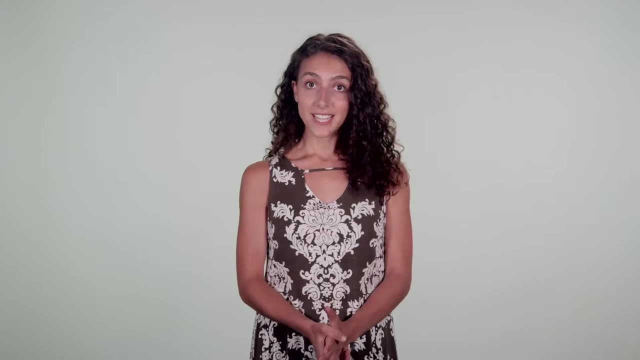 that point-to-point carbon sequestration is an important factor in combating climate change. We have studied all possible causes of carbon sequestration, including the presence of CO2 in our oceans, and we know that carbon sequestration is a rather large factor in the process of carbon sequestration To wisdom and understanding. carbon sequestration is an important part of global economic and economic results. However, carbon sequestration is largely a result of the have-been relation to greenhouse resources and the fact that carbon sequestration 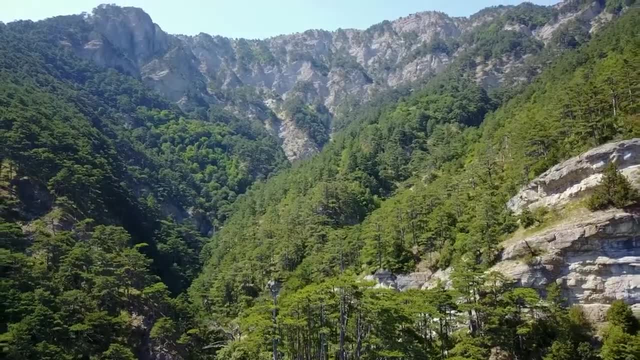 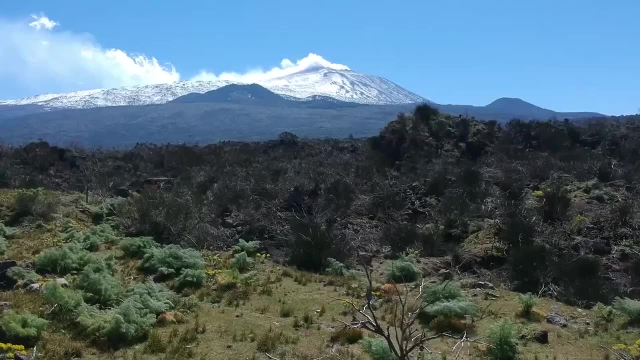 is the most common cause of carbon sequestration in the world. However, we know that every single globe containing a range of different types of trees at different ages, providing old growth and new, They all sequester carbon at different rates. Modeling the carbon cycle will be a mammoth. 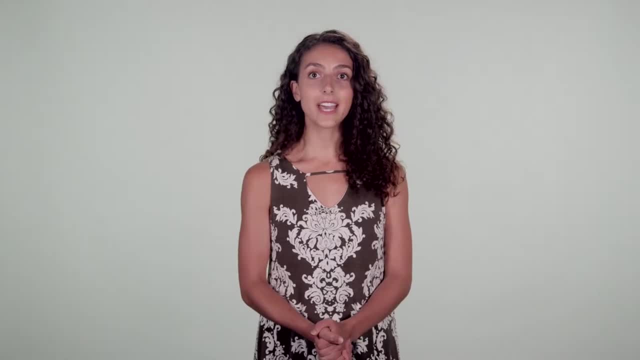 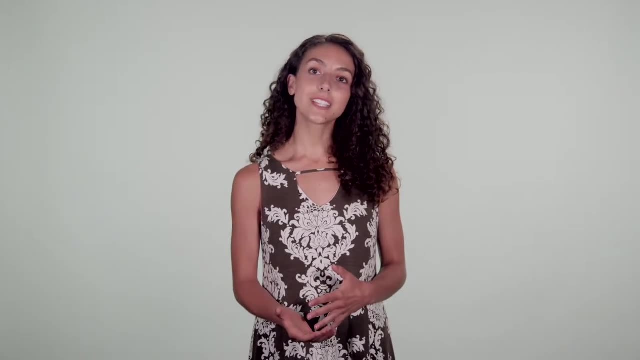 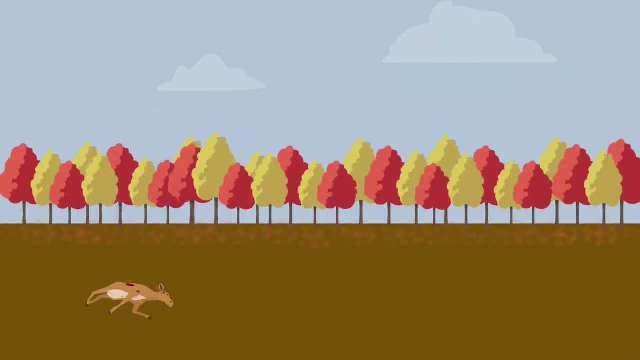 task, and we really hope advances in data modeling and AI will provide these solutions. What needs further examination is how much of the external CO2 emissions will be sequestered into the closed forest ecosystem. Before Mann's intervention, Howard Odom described an ecosystem. 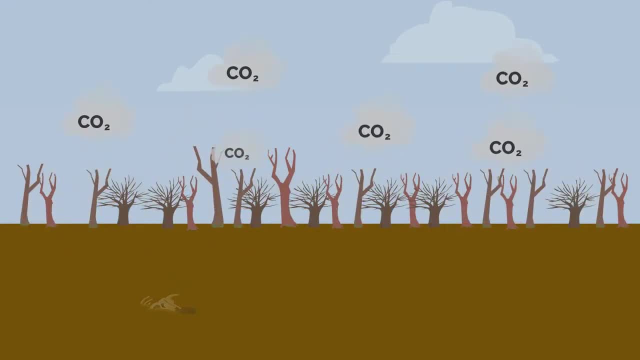 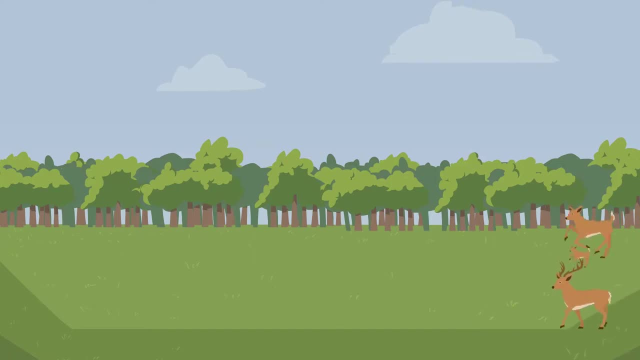 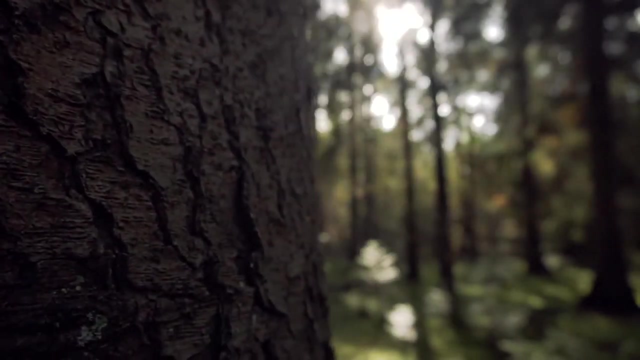 in balance. The carbon released from decaying matter or natural fires is balanced by the growth rate of the forest. But what happens when fossil fuel emissions disrupt this balance? Current studies suggest the extra CO2 in the atmosphere has provided more rapid tree growth. 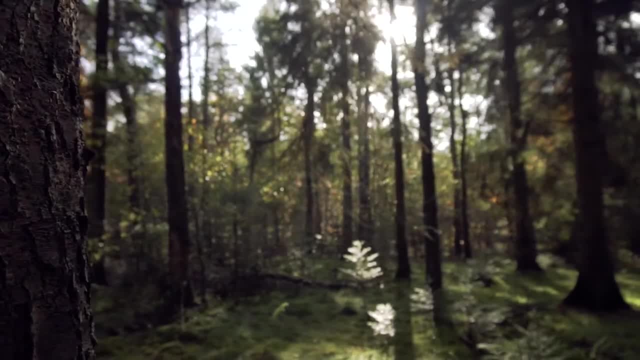 In the last 50 years, forests are taking in more CO2.. This is because the CO2 emissions in the atmosphere have increased. This is because the CO2 emissions in the atmosphere have increased. This is because the CO2 emissions in the atmosphere have increased. This could be a cyclic change. However, in no 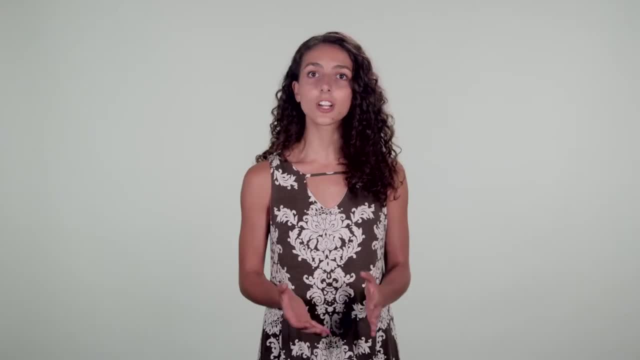 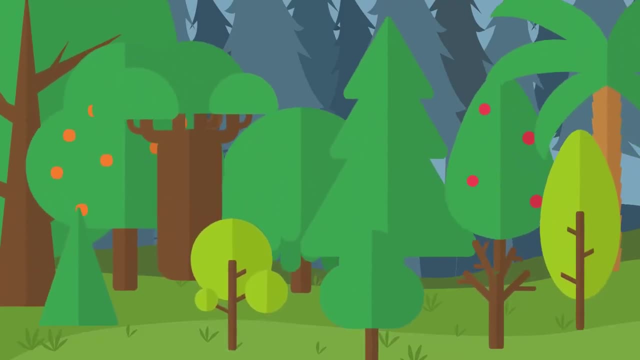 period in the past? does any data suggest this has ever occurred on a global scale? So is it good for combating climate change if the trees are growing at a faster rate? Unfortunately, that may not be the case If trees are living shorter lives due to the 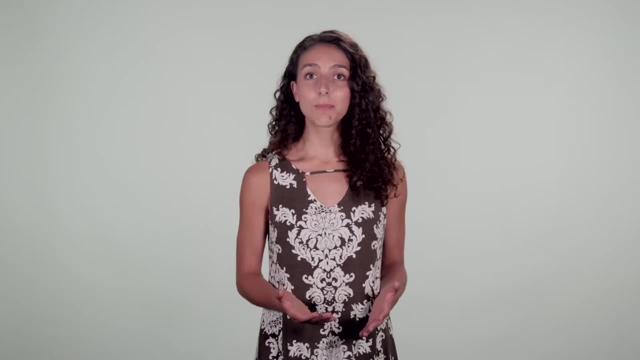 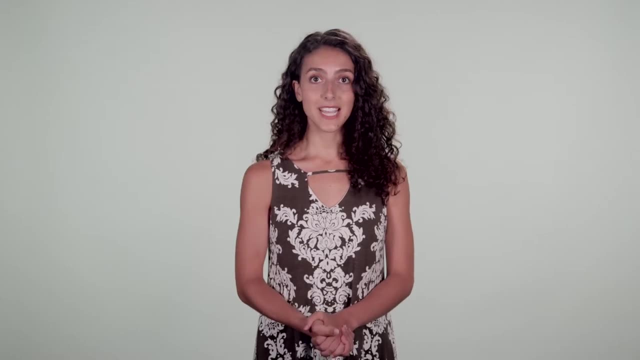 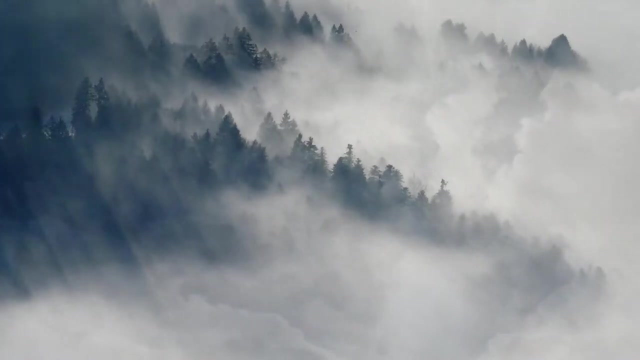 increased growth rate. current models have not included the possibility that soil fertility may fall. What happens when this fertility falls below the limit? The climate changes in our climate and the changes in a forest's ecosystem still require further studies, but there does appear to be a strong connection As with climate science the full